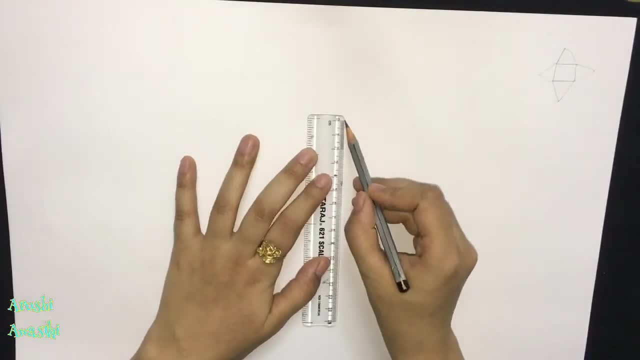 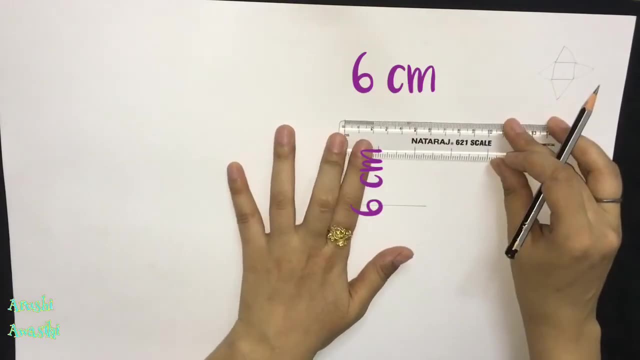 Toh kyunki hum banara rahe hai square pyramid, toh of course sabse pehle mein ek square banana padega hai. na Toh, main yaha par ek square banara rahe hu, jinki measurement mein 6 cm leh rahe hu. 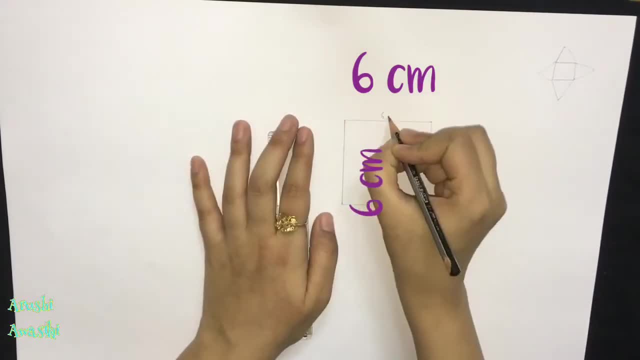 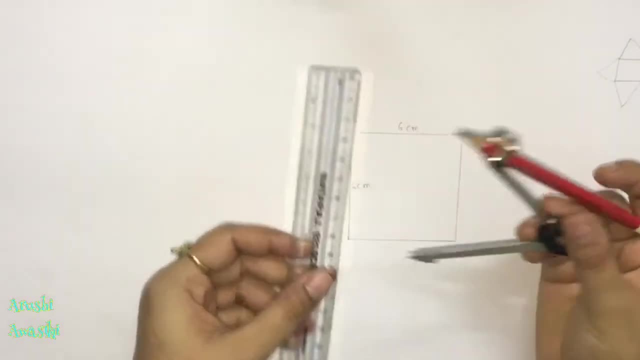 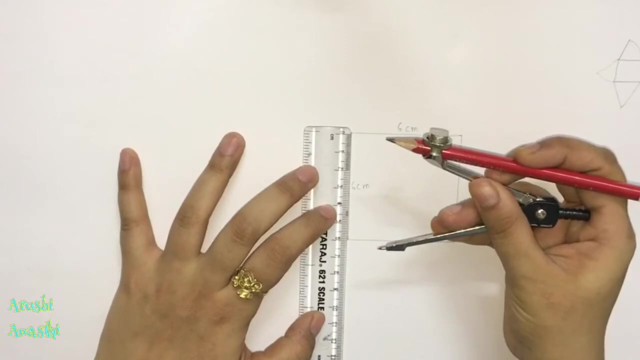 Toh 6 cm length and 6 cm breadth. So, guys, here comes the fun part. Now we have to make triangles. Toh triangles banane ke liye mein yaha par compass leh rahe hu. aur aapko scale ki, madad, se compass, se utne hi measurement tak ka khulna hai, jitne ki humne square banaya hai. 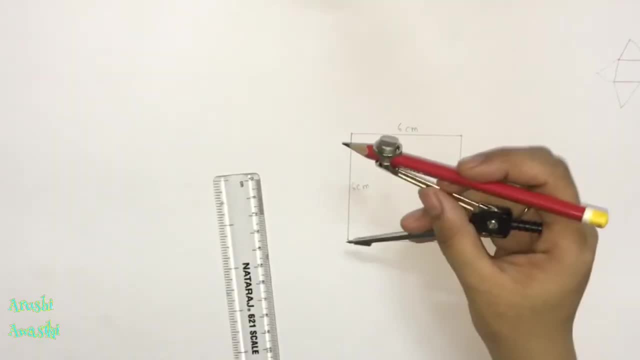 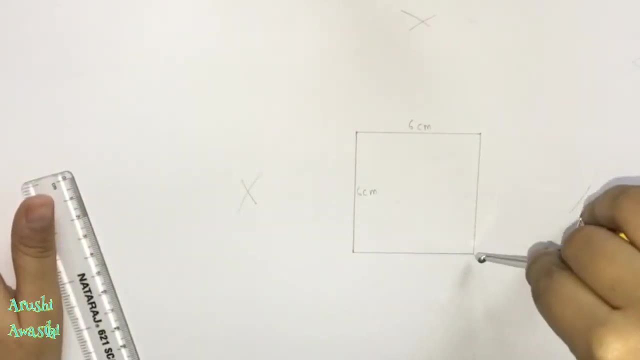 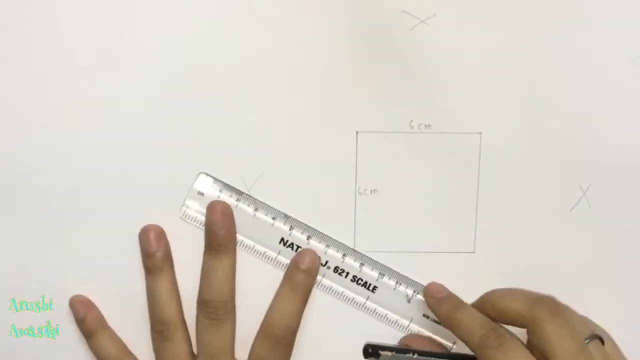 Jaise ki maine 6 cm ka banaya tha, toh I am taking the same measurement as 6 cm. And then we have to make two arcs like this. And why I have chosen this method? Because isse humara ji triangle hai bohot, hi accurate banega Kalti ki kuch chances hi nahi hai. See, 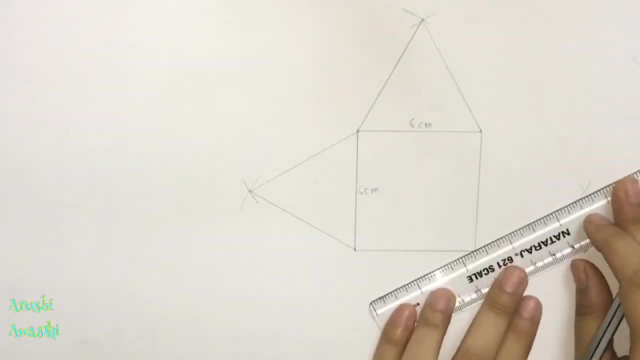 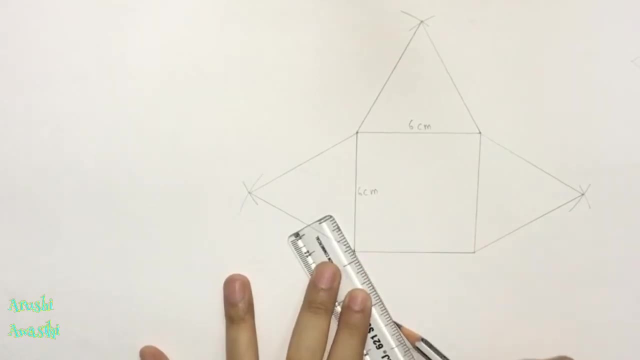 But if in case kisi bhi reason ki wajah se aap is method ko use nahi kar pae, so not to worry, stay tuned, mein aapko aake batahongi, ki iska alternative kya ho sakta hai. 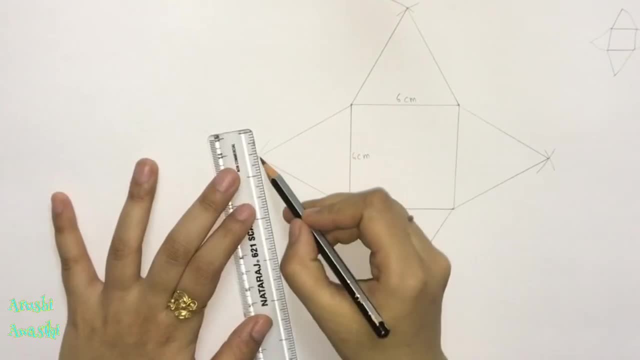 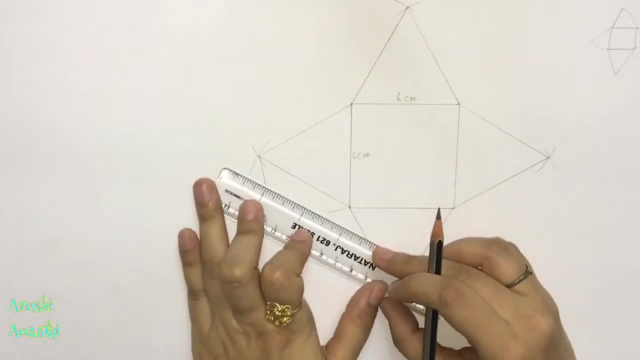 Now we have to take 1 cm and do one parameter extra measurement. And yes, jen logo ne meri purani shapes ki video dekhi hui hai. unko definitely pata hoga, ki me inka kya karne wali hu. 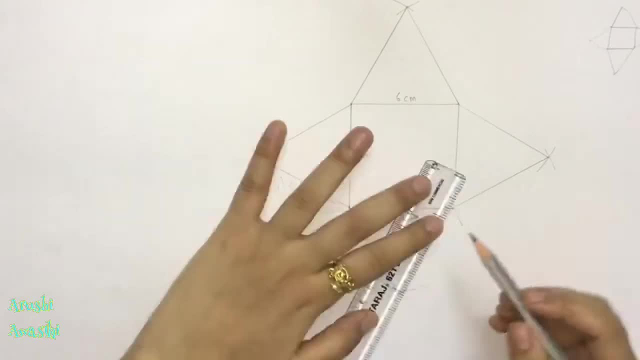 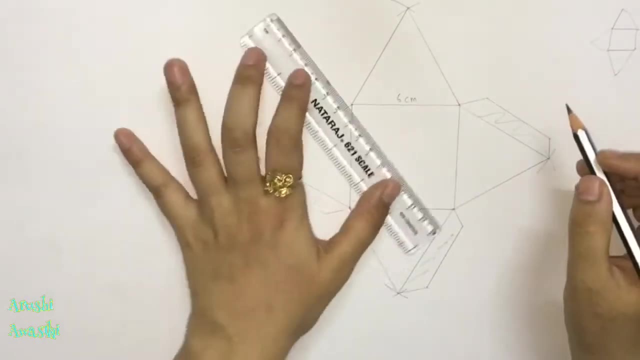 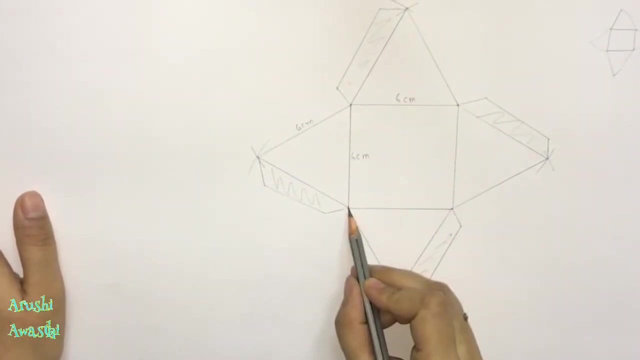 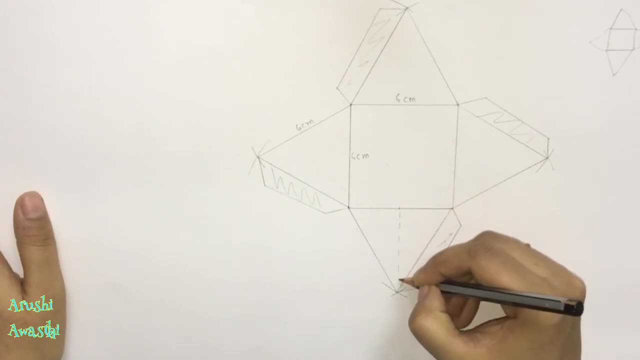 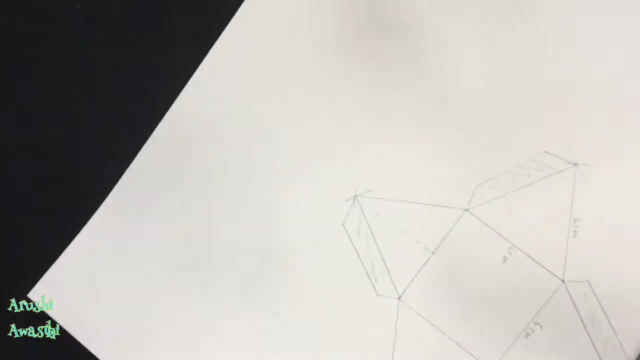 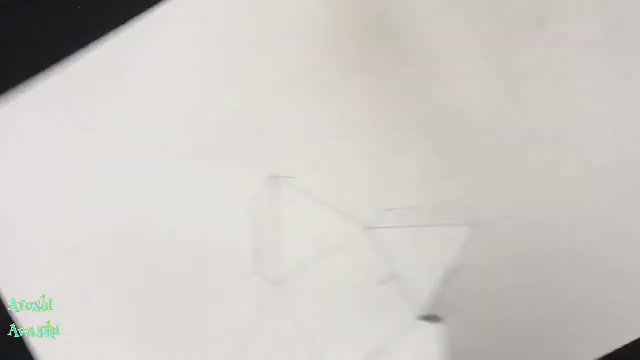 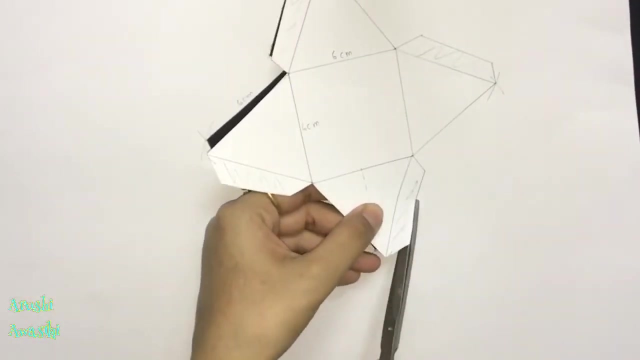 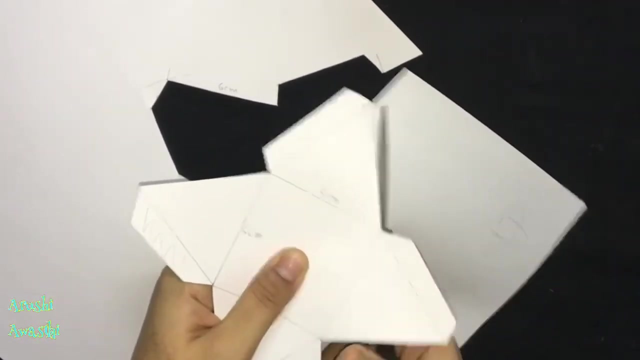 I will tell you. so here we have taken 6 cm, so you can measure it by half. that means 3 cm, and then you can draw a line like this and you can make your triangle like this: music ta-da. it's ready, now we have to fold it.